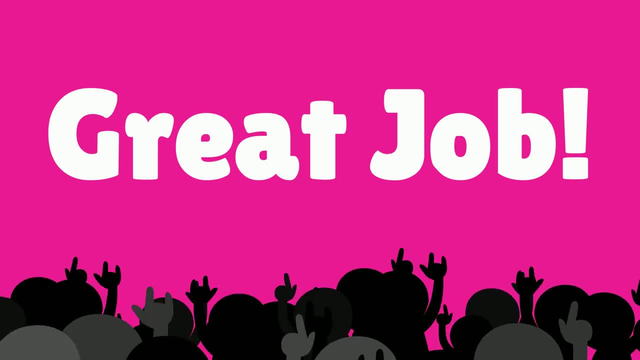 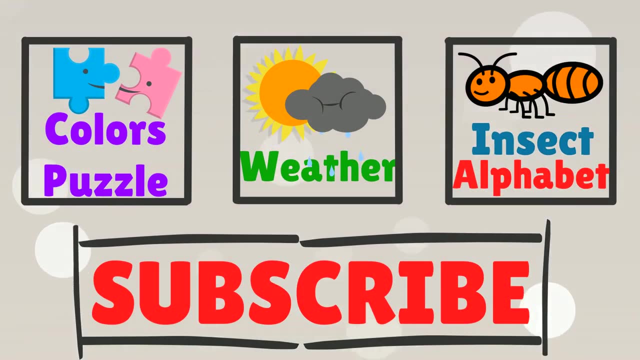 Great job, Yeah, Thanks. 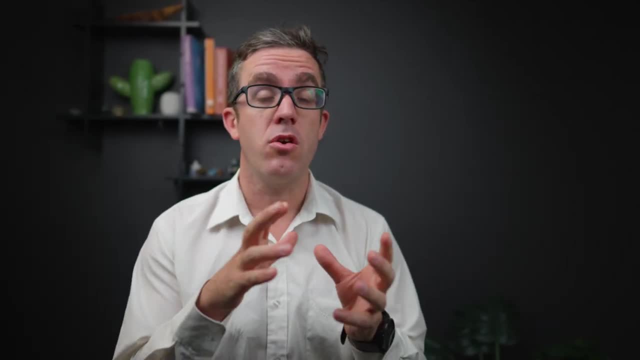 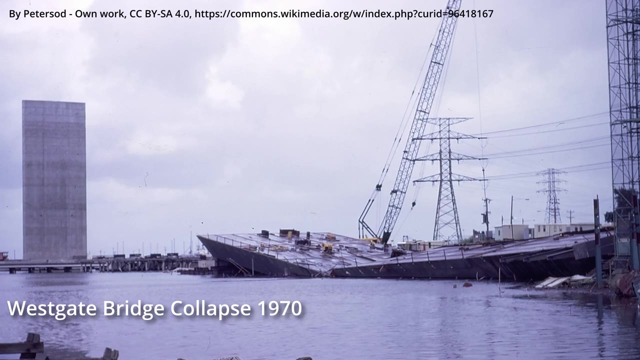 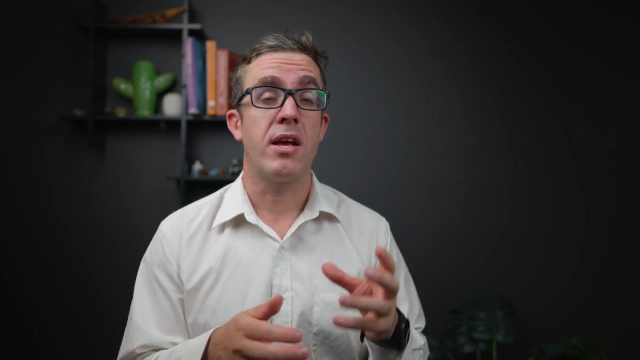 The design of steel connections is literally the most important thing that you can look at in any structural steel design. It can literally make or break your structure and many people overlooked it and has led to disastrous consequences. So I'll be going through the basics of steel connection design to make sure that you can make the right decisions and things. 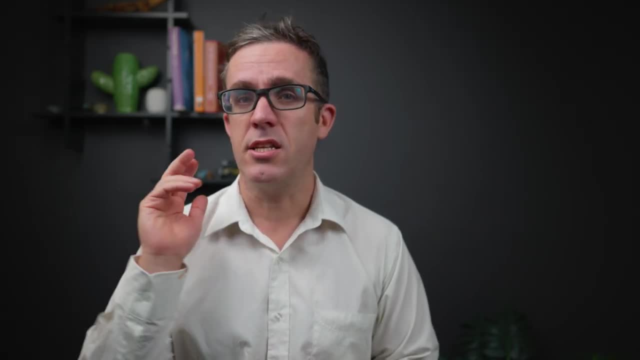 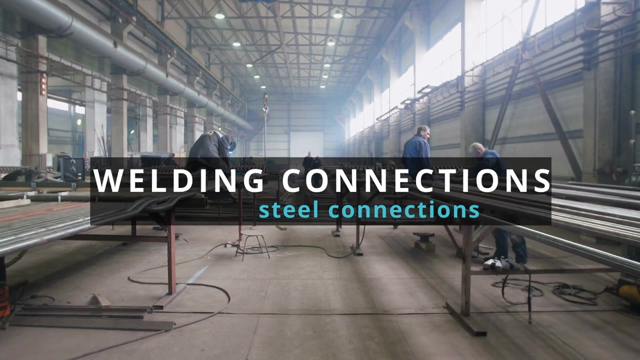 that you should look out for. My name is Brendan, your structural engineer. Now let's get into it. So what type of connections can you have in a steel structure? You can either have welded connections or bolted connections. Welded connections are quite easy to understand. 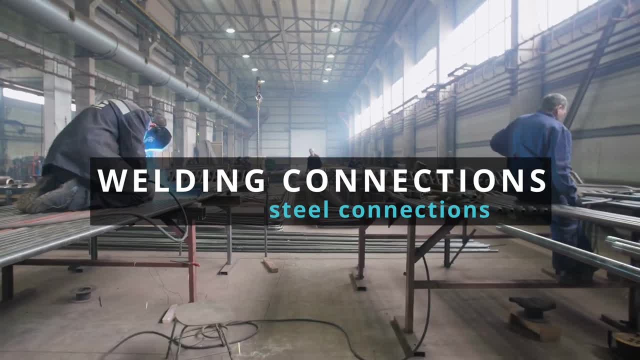 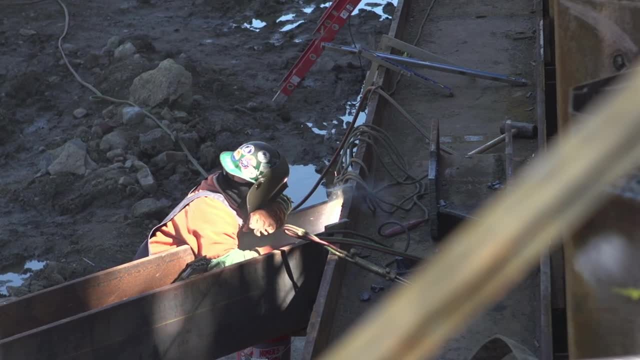 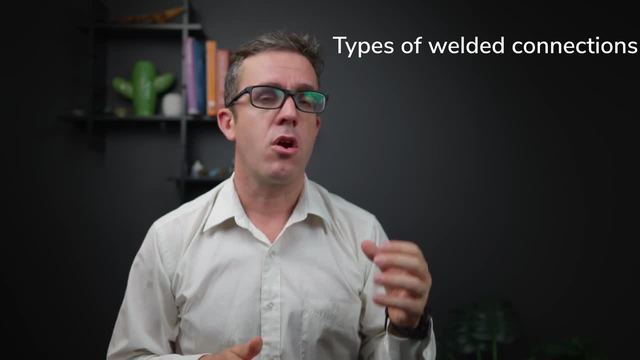 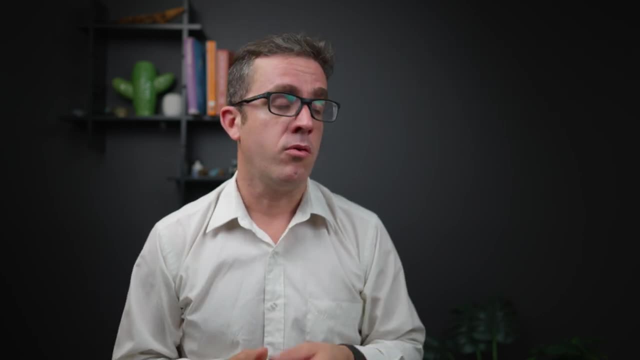 There's also two main types of welds that you may be looking for. You either got a full strength butt weld, which is FSBW, or a continuous fillet weld- CFW- So the full strength butt weld. you've got two bits of steel, you made a chamfer and you butt weld them together to get a full. 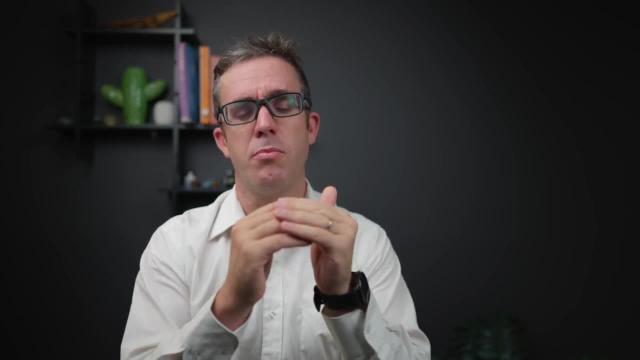 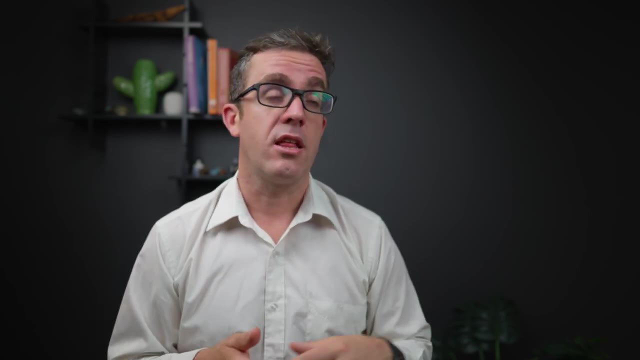 strength connection, Whereas a fillet weld you're potentially connecting two plates together or two areas together and you're just filleting locally in that area. So you can have different sizes of fillet weld. So you can have a six CFW, a four CFW, three CFW, 10,, 20, whatever's. 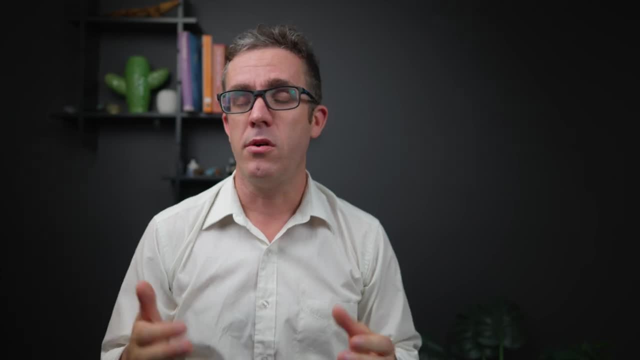 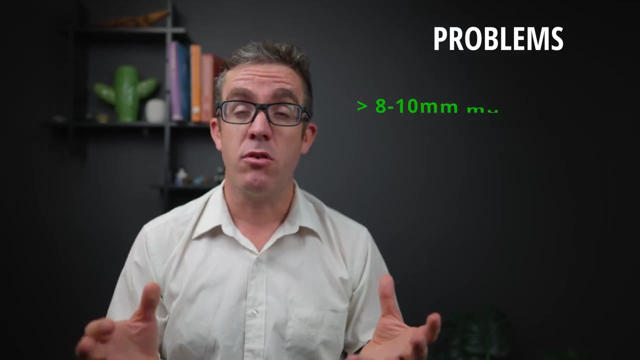 load you need a hundred millimeters of weld. If you're looking to resist high forces, you can just put a bigger fillet weld, So an eight fillet weld, 10 fillet weld or even bigger. There's a couple of problems with that And if you go more than about an eight or 10 weld,